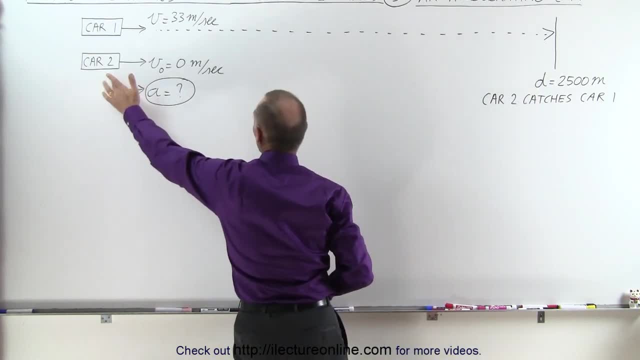 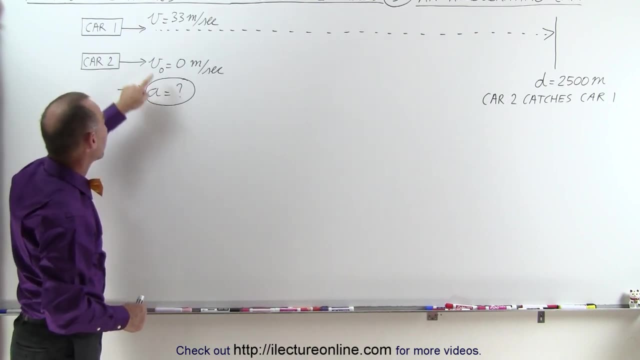 reaches a distance of 2,500 meters, the second car will have caught the first car. The question is: what is the acceleration necessary for the second car in order to catch the first car after 2,500 meters? So what we can say in this case is that the time spent for the first car and the 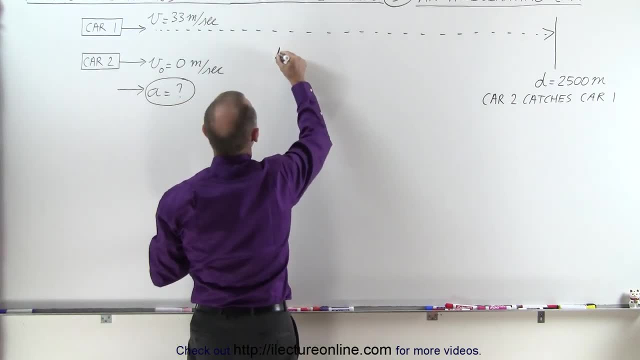 time spent for the second car is the same. So t1 is equal to t2, and we can also say that distance covered by the first car must equal distance covered by the second car, which in this case is going to be 2,500 meters. So if that's the case, what we can do is 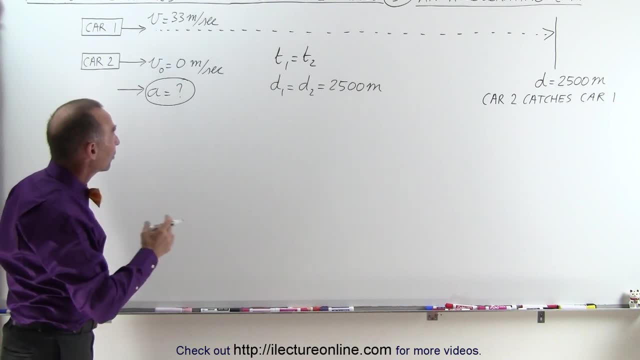 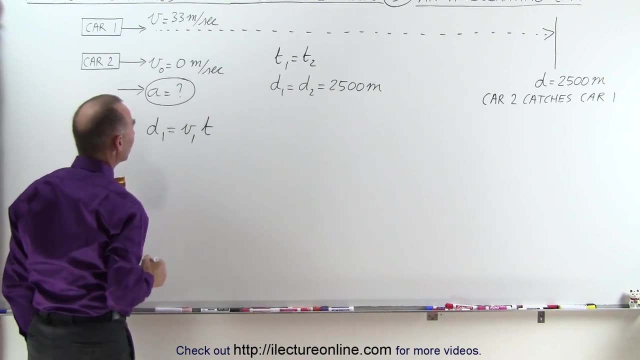 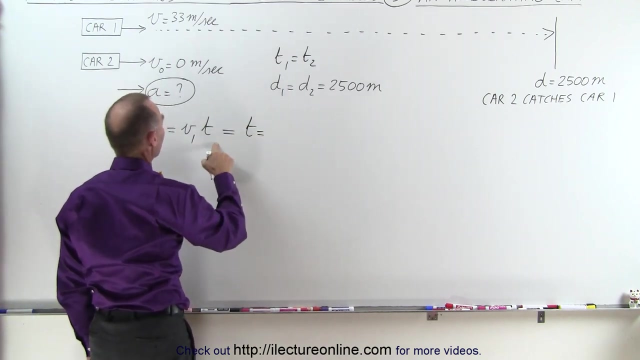 we can solve for the distance traveled by both cars separately. We can say distance 1 is going to be equal to the velocity of the first car times the time spent, and we know the distance and we know the velocity, which means in this case we can actually solve for the time, The time. 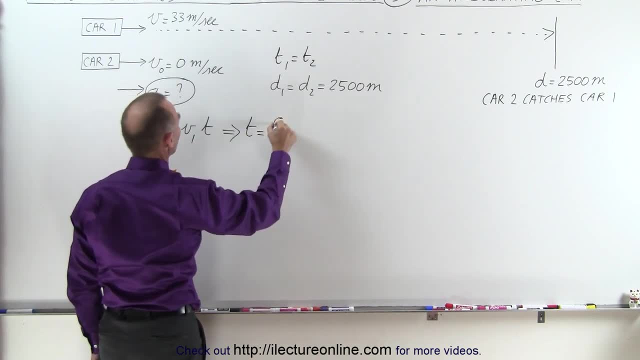 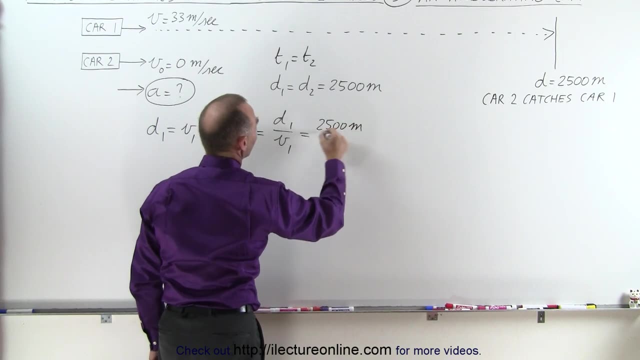 let's put an arrow there. the time is going to be equal to distance 1 divided by velocity 1.. So distance 1 is going to be 2,500 meters and velocity 1 is going to be 2,500 meters. 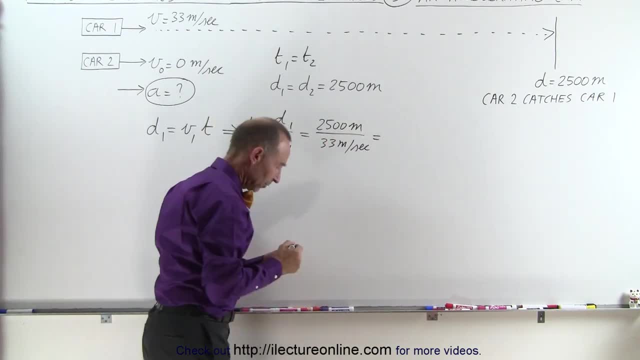 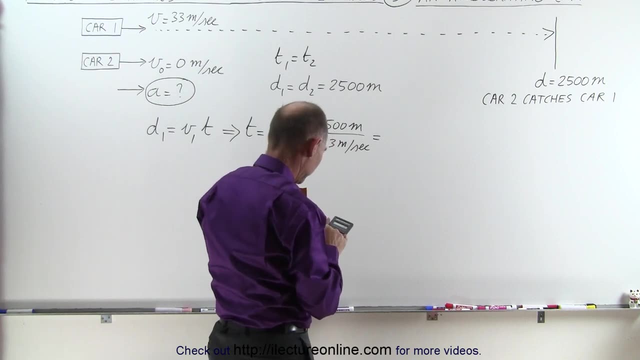 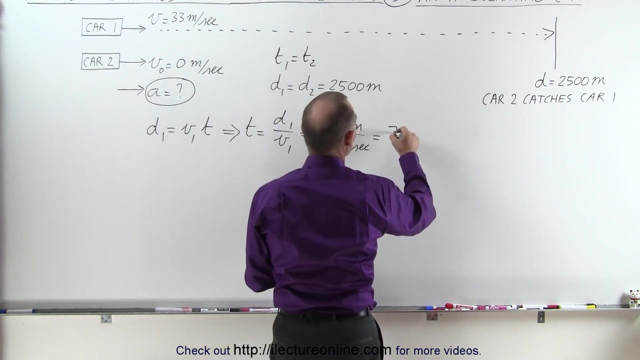 So in this case we're going to know how long it's going to take for the car 1 to get there and also for car 2, because the time will be the same. So 2,500 divided by 33 is 75.75.. So 75.758. 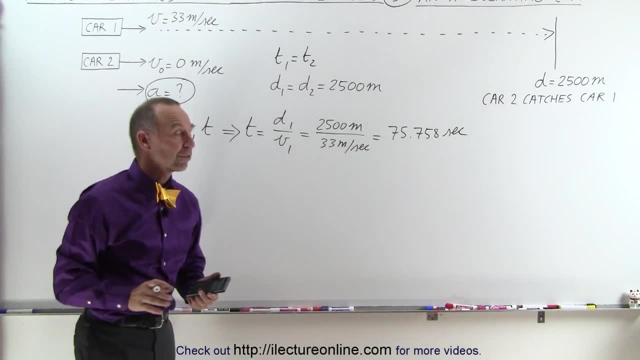 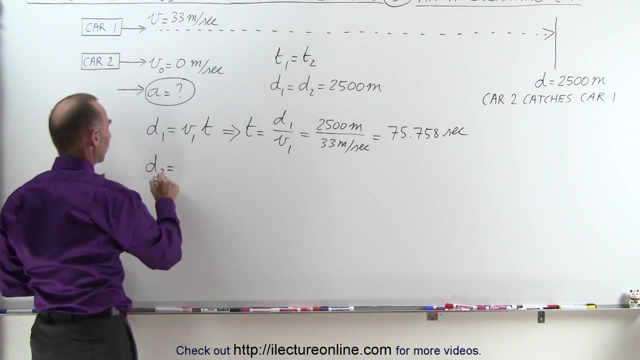 seconds. So that's the amount of time it takes for both cars to get to a distance of 2,500 meters. Then distance 2, since there is only an acceleration- there's an acceleration here- we can say that distance 2,. 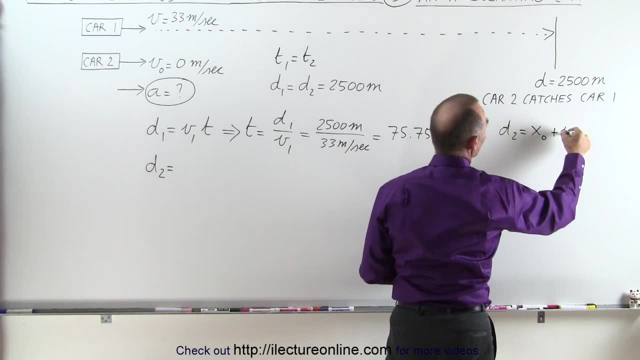 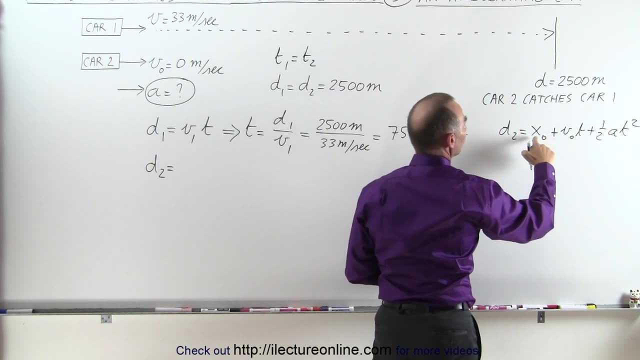 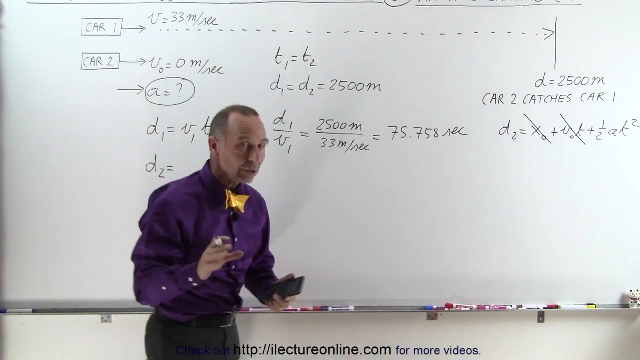 d2, is equal to the initial distance plus the initial velocity times time plus one-half the acceleration times, time squared. But since there's no distance traveled at time equals zero, this goes to zero and there's no initial velocity for car 2, so therefore it only depends on the 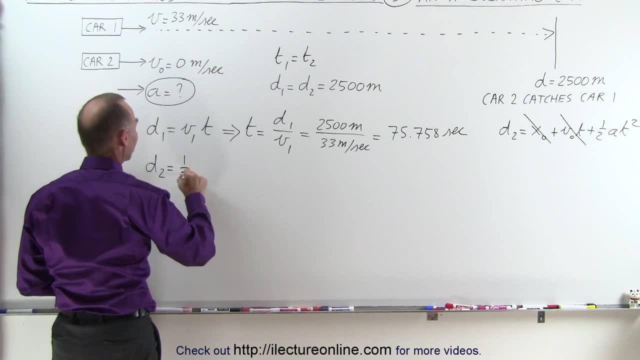 acceleration term. So distance 2 is going to be equal to one-half the acceleration times, the time squared. Now we know what the time is because it's the same for the time for the first car, and we know the distance because that's the same for as the first car. so we could solve this.